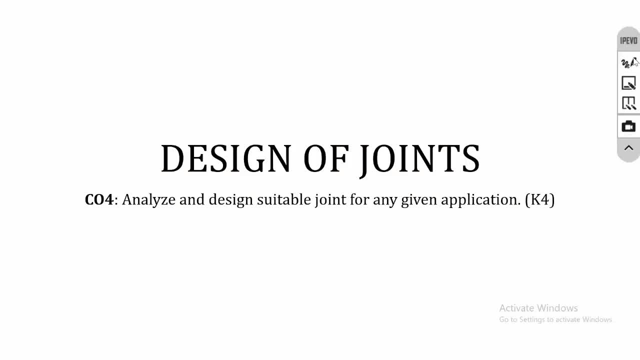 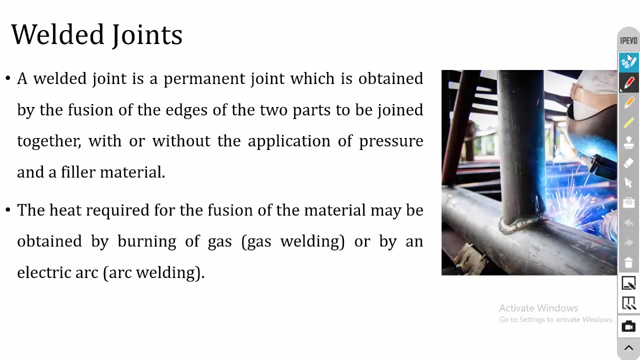 In this lecture I am going to start the fourth CO, that is design of joints. So the CO statement is: analyze and design suitable joint for any given application. So in this unit we are going to deal with the design of welded joints, then reverts and design of bolted joints. So first we will start with design of welded joints. So first, what is welding? So welding comes under a permanent joint where the two materials are jointed by the fusion of edges of the two parts. So fusion means it is the metallurgical relation between the metallurgical bond between the parent material. 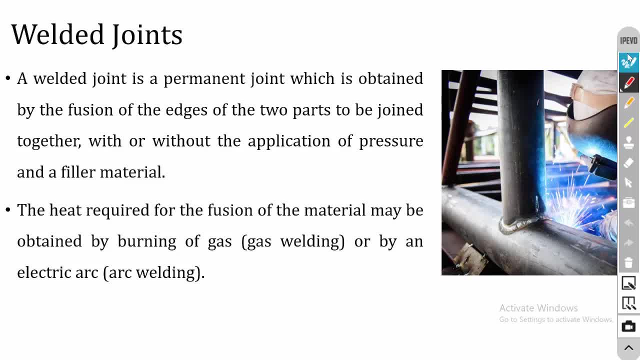 So in this welding, in some case the welding is carried out with the help of filler materials and pressure, and in some case the welding is carried out without the pressure. In case of gas welding, the heat required for the welding is generated by burning the gas, and in the case of arc welding, the heat is produced by electrical arc. 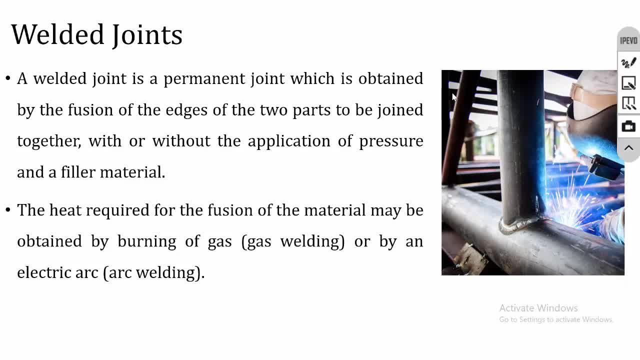 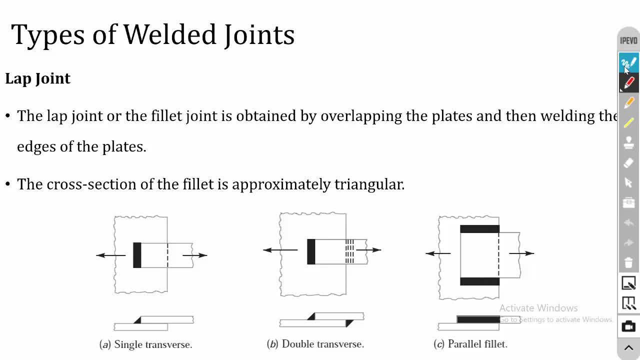 So I am not going to deal what is welding in depth because you have already studied welding in manufacturing technology. Types of welding. So first one is lab joint. In lab joint the two plates are kept one over another and the welding is carried out. So here the cross section of the weld is approximately a triangular section. 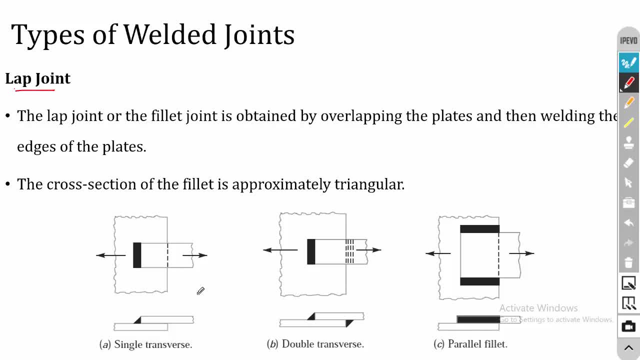 There are three types of weld. types of lap joints are there. The first one is single transverse weld. so in this the weld is carried out in the transverse direction and in only one side of the plate. In case of double transverse weld, the welding is carried out in transverse manner and you can see that. 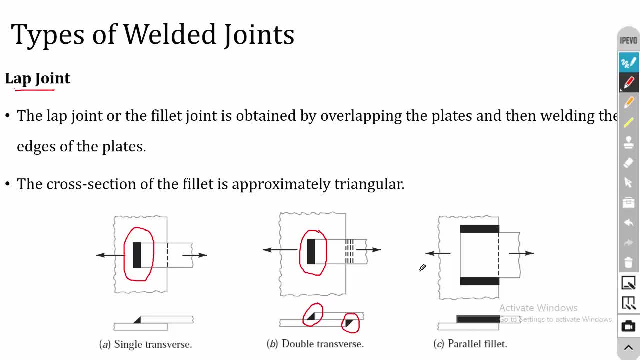 the welding is carried out on both the sides of the plate. In the case of parallel fillet weld, the welding carried out in a parallel manner. ok, so the load is applied here and the welding is carried out in the parallel direction. So these are all the three types. 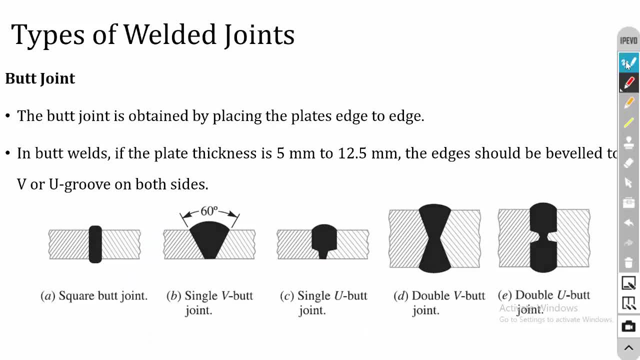 of Lap joints Then butt joint. so in butt joint the welding is carried by placing the plates in a edges to edge manner. So if the thickness of the plate is less than 5 mm, then there is no NEED to prepare the edges. If the thickness of the weld is greater than 5 mm, then the edges should be beveled. 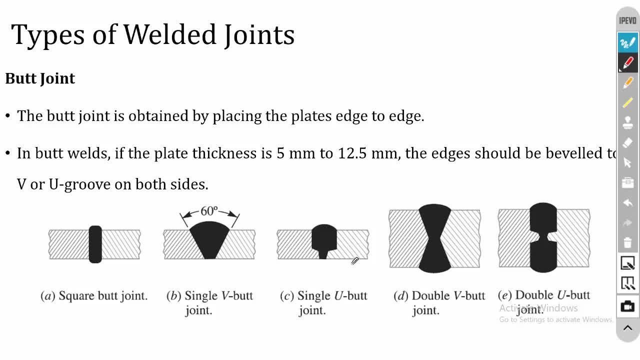 So whether we can go for V butt joints or whether we can go for U butt joints, So these are all the different types of butt joints. So first one is it's a square butt joint. The second one is it's a single V butt joint. 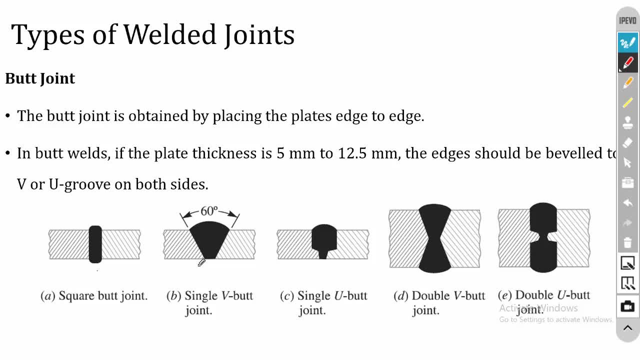 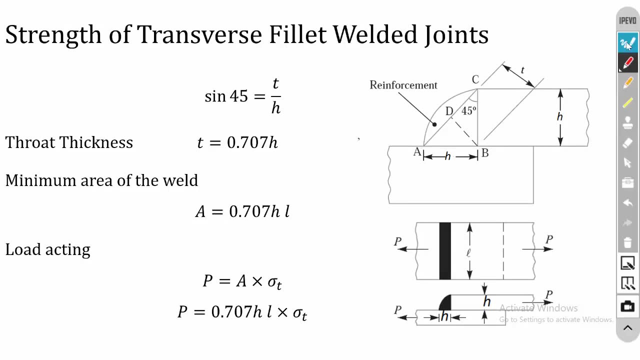 So the plate is bevelled in only one side and here it is U butt joint. If the thickness is high then double V butt joint or double U butt joint is used. Strength of transverse fillet welded joints. So in the CO we are going to design the strength of the welding. 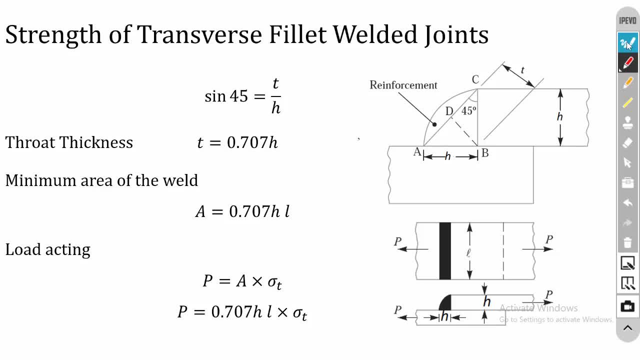 So we have to analyze the stress acting on the welding. First I have considered The transverse fillet weld. So you can see that this is the weld region A, B, C and D. So I have considered triangle here- A, B, C and D and the inclination is 45 degree. 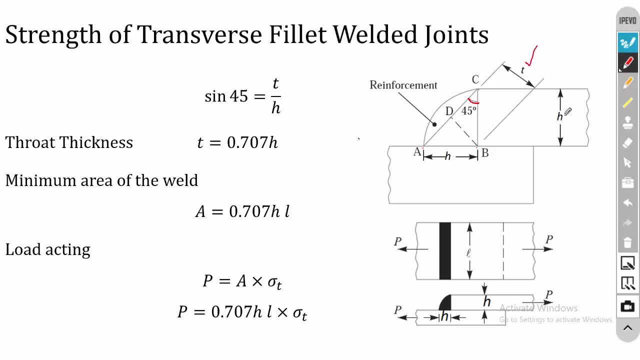 So here T is the thread thickness of the weld and H is the weld thickness. So there is a difference between thread thickness and weld thickness. T is the thread thickness and H is the plate thickness. So if you take sin 45, sin 45 is equal to T divided by H. 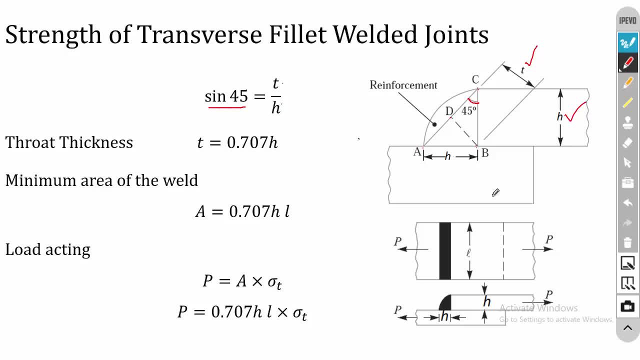 So consider the triangle C, D and B. So sin 45 is equal to opposite side by adjacent side. So here the opposite side is T and the adjacent side is H. So the thread thickness T is equal to sin 45 into H and sin 45 is 0.6.. 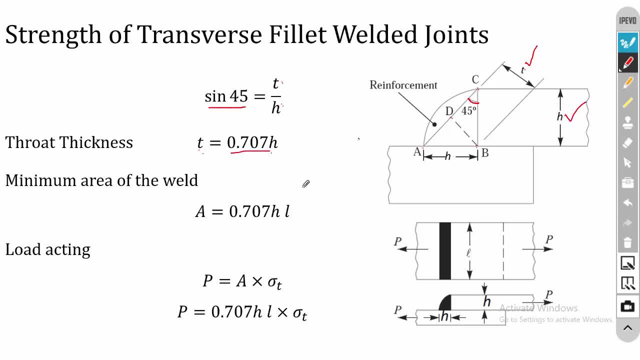 0.707, so t is equal to 0.707 into h. then to find the area of the weld, the area of the weld a is equal to, so this is the cross section and this is the length. so the weld is carried out throughout the length and the length is l, so it's t into l and in the place of t i have replaced. 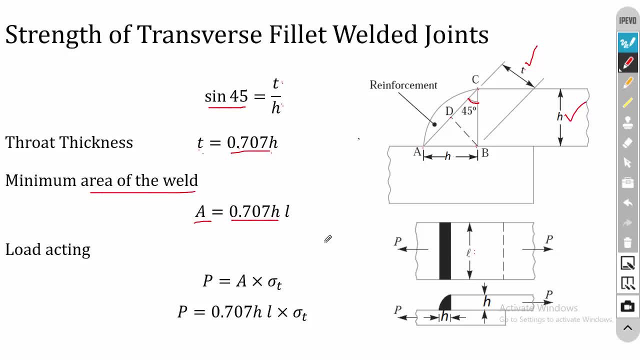 with 0.707 into h. okay, so in the three-dimensional it will be like this: okay, so this is t and this is l. so the welding area is t into l. t is equal to 0.707 h into l. so now the load p is acting. 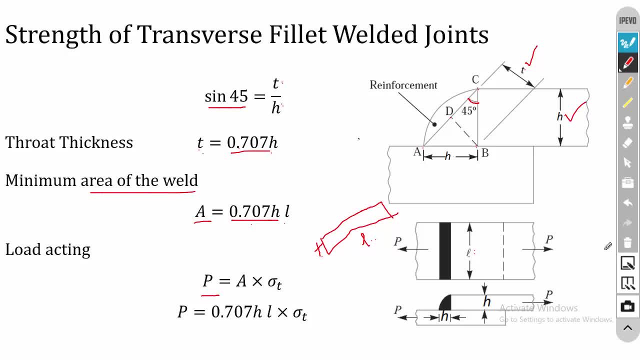 in a transverse manner. so if the load p acts like this, then a tensile stress will be acting on the welder. okay, so, and the area a is resisting the tensile stress. so load is equal to area into stress, load p is equal to area. we have already calculated t 0.707 h into l and sigma t is the tensile stress. 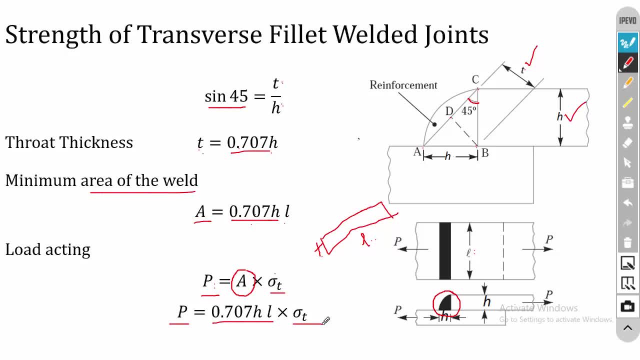 acting on the weld. so to find the weld thickness, then we can use this equation, that is: p is equal to 0.707 h into l, into sigma t in the case of single transverse fillet weld. so here p is the load acting, h is the. 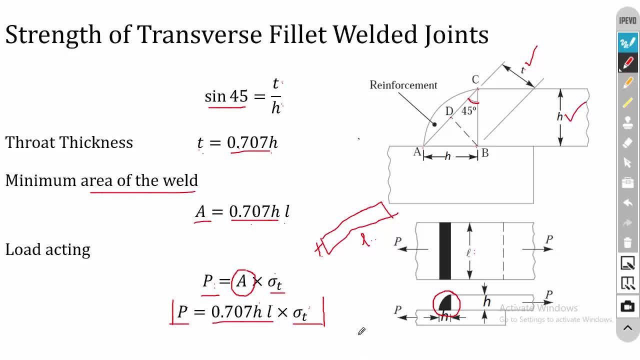 plate. thickness l is the length of the weld and sigma t is the tensile allowable tensile stress of the weld material. so to find the weld thickness we know the load value, the length of the plate and the sigma t of the weld material. so if you know the remaining data then we can find the 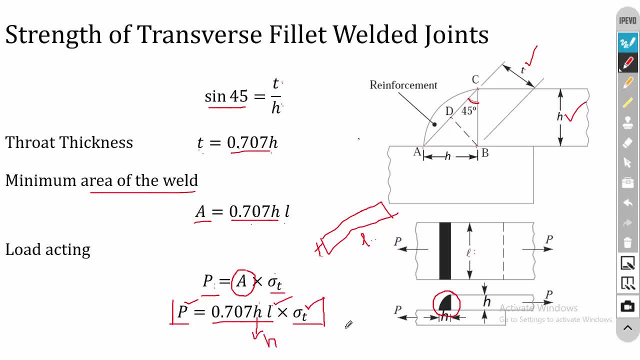 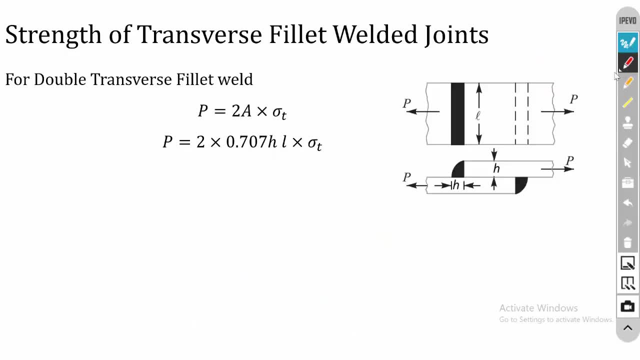 of h, that is the plate thickness or the weld thickness. So this is for a single transverse fillet weld. In the case of double transverse fillet weld the welding is carried out on both the sides of the plates. So it is 2 times the area. so I have multiplied 2.. 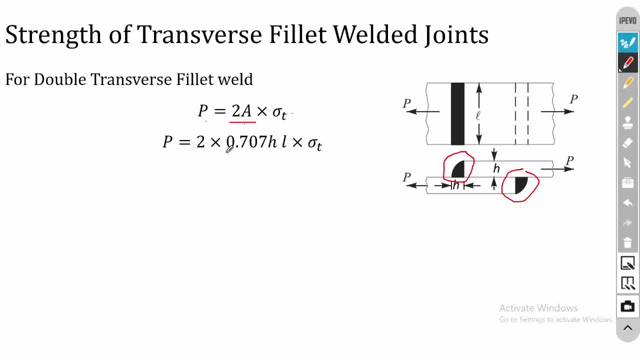 So P is equal to 2a into sigma t and we know that a is equal to 0.707 h into l. So this is for a double transverse fillet weld. If in the problem the double transverse fillet weld is given, then you have to use this equation. 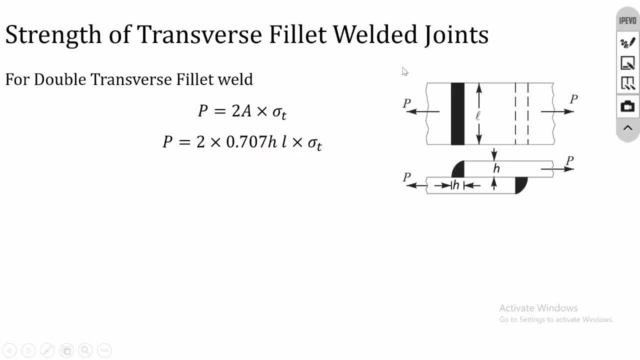 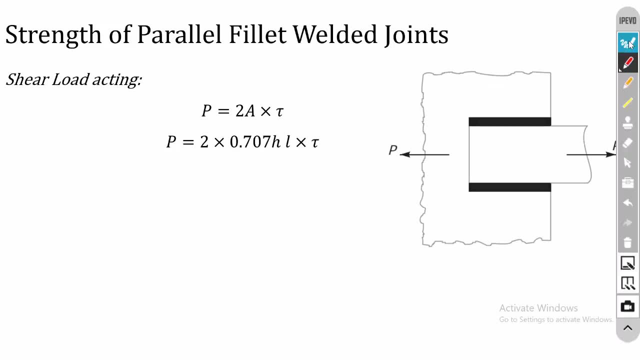 to find the h value. And this is parallel fillet weld. So in the case of transverse fillet weld, tensile stress will be acting on the welding. In the case of parallel fillet weld, you can see that when the load is applied like this. 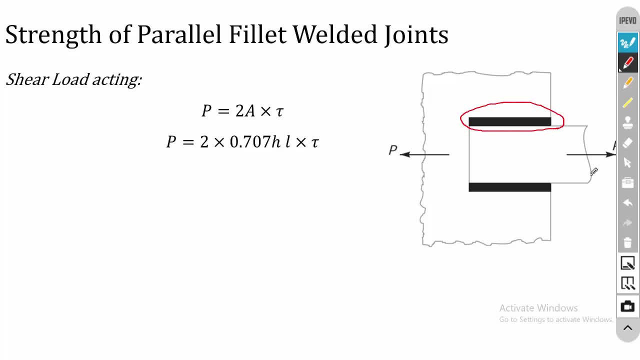 then shear stress is acting on the welding. So if the welding is carried out here, then the tensile stress will be acting because it is perpendicular. But if it is a parallel fillet weld means, then shear stress will be acting And the equation is same, that is, P is equal to. here the welding is carried out on two. 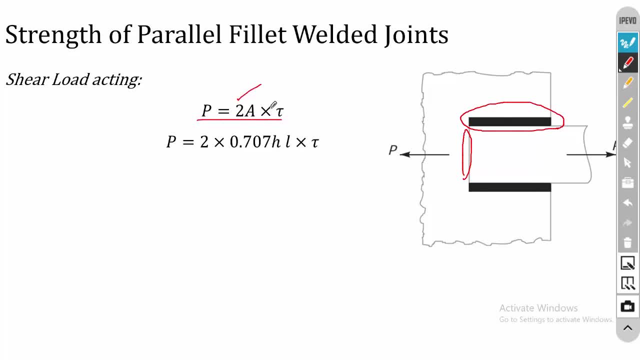 sides. So that is why I have multiplied 2 here. it is 2a into tau. it is not sigma t, because here the shear stress is acting. So P is equal to 2 times 0.707 h into l. this is a and tau. 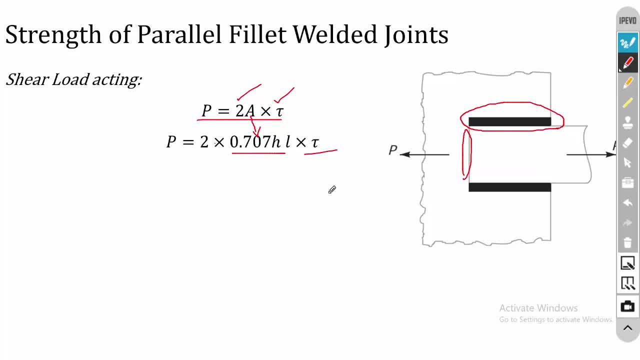 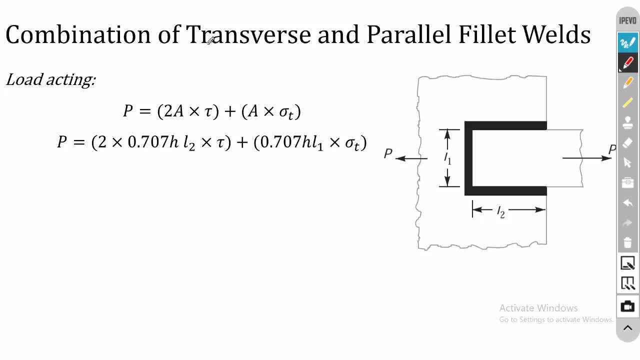 So this is for a parallel fillet weld. Then, finally, it is a combination of transverse and parallel fillet weld. First, consider the parallel fillet weld. two parallel fillet welds are considered, So it is 2a into tau. 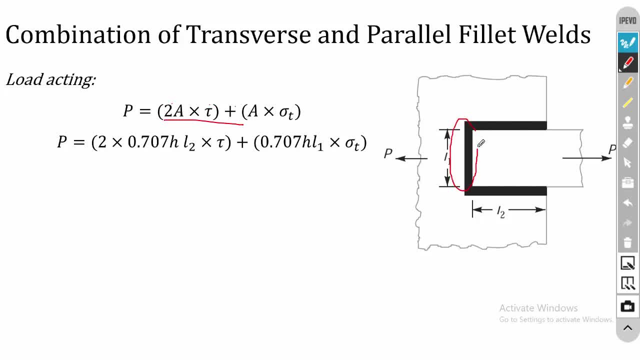 Then plus Here another transverse fillet weld is considered, So it is a into sigma t, because the transverse fillet weld is subjected to tensile stress. Further we can substitute the value for area- So P is equal to 2- into 0.707, h into l2 in the case of parallel fillet weld, because for 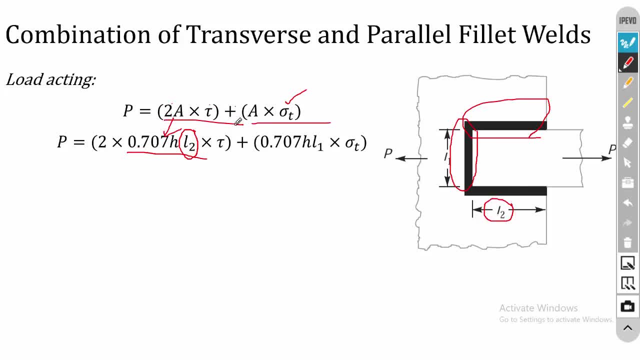 parallel fillet weld, the length is l2.. Then plus, So this is a- A is 0.707 h into l1 in the case of transverse fillet weld, because the length of transverse fillet weld is l1 into sigma t. 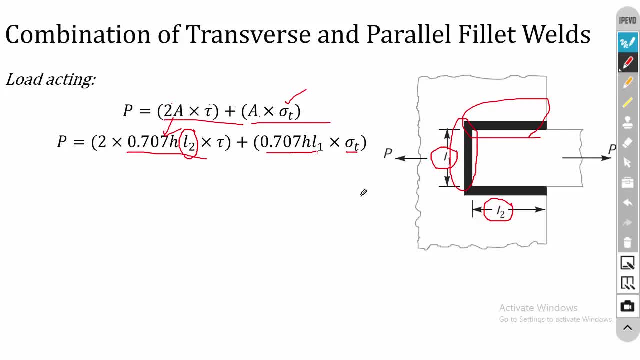 So this is for a combination of transverse and parallel fillet weld. So in the problem they will give the diagram, they will give the load acting and from the load acting and the stress value we have to calculate the thickness requirement of the weld. 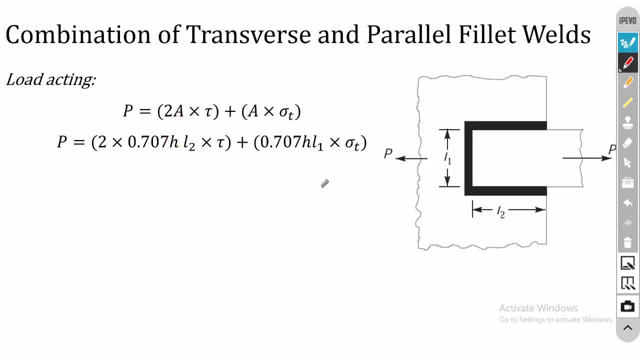 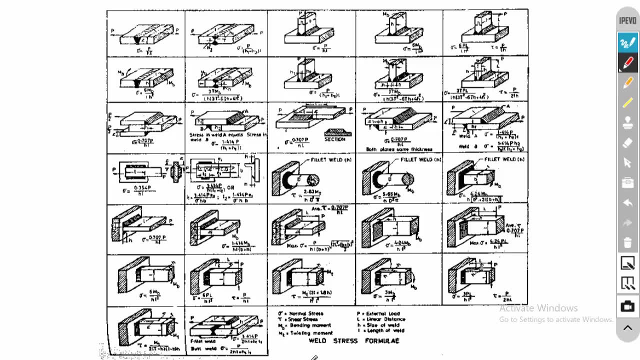 Ok, So this is our objective in this CO, And all these equations, what I have derived, is in the data book, page number 11.3.. So you can select the appropriate drawing based on our given problem and from the drawing we can take the formula, we can substitute the values and we can calculate the weld size.